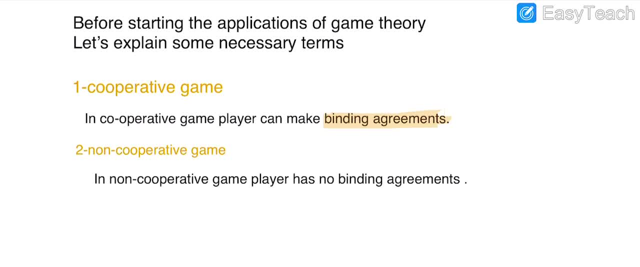 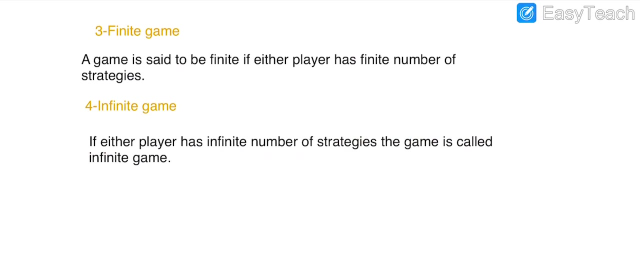 is opposite of cooperative game, in which player has no binding agreements. and what's that term? third, finite game. and infinite game? actually finite game- in which player has actually finite number of strategies which the player is going to adopt for the starting of the game and how many strategies the player can. 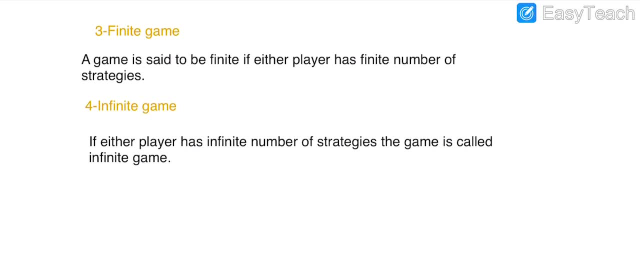 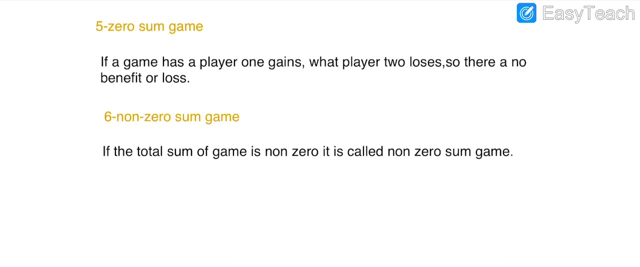 be a top. either player is in the position to adopt finite number of strategies, it is called finite game, and if the players is in the option and the position to adopt infinite number of strategies, it is called infinite game. next one is: what is zero-sum game and non zero-sum game? these two terms are these: 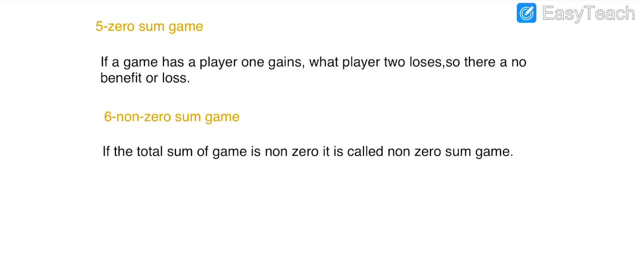 two terms are very important, on which we are going to do the numericals in the next. for example: first we discuss what is zero-sum game if the player zero-sum game actually, when such type of situation in which a player what's gain second player actually is. 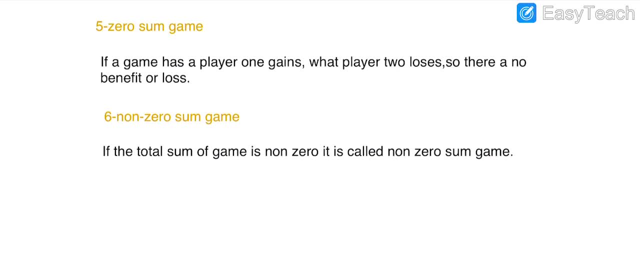 same loss. for example, one player gets 2% benefit. second case is losing 2% of benefits. it mean overall situation will be 0. it's mean benefit of one player is equal to the loss of another player. this is the situation of four balanced mean worse will, with a profit of 1% that will. 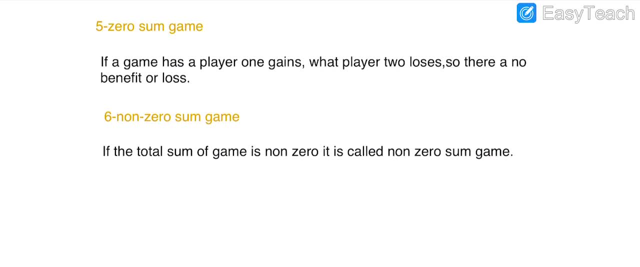 be the loss of another person with greater benefit of other players. so this is the same principle we will discuss in future videos. So it's called zero-sum game. There will be nothing obtained in this game. And what is non-zero-sum game? Non-zero-sum game is if the total sum of the game is non-zero. 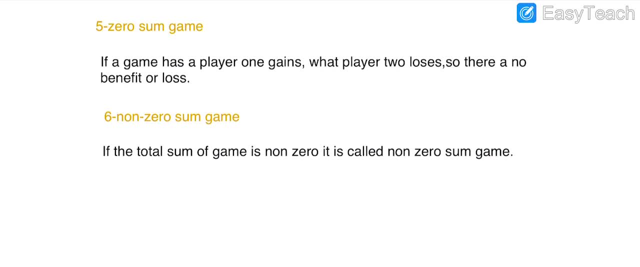 I mean like the zero-sum game, where benefit and loss was equal. But in this game, benefit and loss is not equal. Maybe in some situation loss is greater than benefit, or in some situation benefit is greater than loss. Any situation can happen, but it depends upon the situation of the market according to which players are going to play. 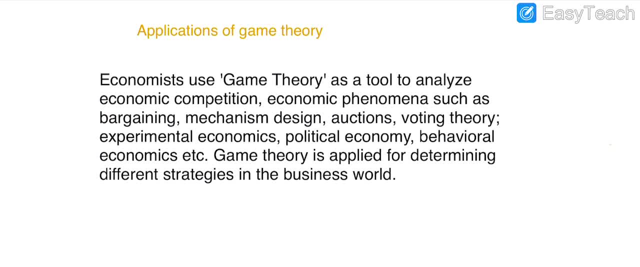 Let's discuss the applications of the game theory. Actually, game theory applied in many fields, not only economics, in real life, in political economics, in psychology, in sociology. in economics It's actually, it's a wide concept And if we see the game theory in the field of economics, how economists use this into the real life, 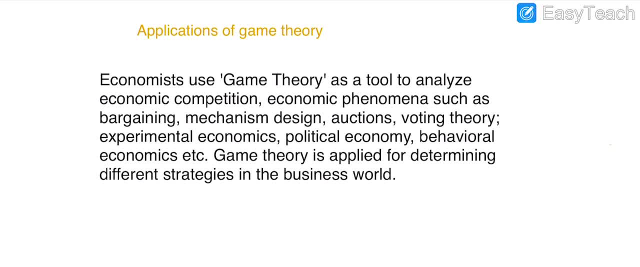 Actually, game theory is a very interesting topic And when the firms are going to decide about their production, about their profit, about their loss and how they have to play into the economy, how to have they play into the competitive market, they actually utilize or they take help from the game theory. 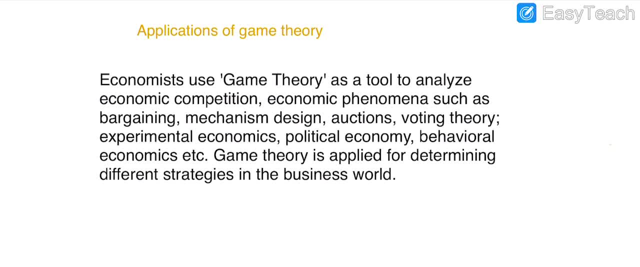 And economists use game theory as a tool to analyze. I see economic competition, economic phenomena such as bargaining Mechanism, design options for voting theory, experimental economics, political economy, behavior economics, And actually is this applied for determining different strategies into the business world? 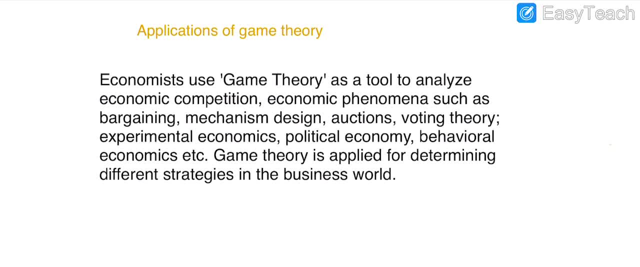 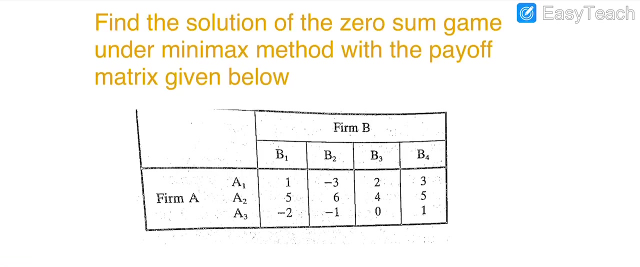 Game theory is a wide concept and that is going to you use the different fields and we can understand the concept by solving different types of numericals. let's start numericals on different strategies of game theory, so you clearly understand the concept of game theory. first, we see that as i tell you about the zero sum game, so we see how the zero 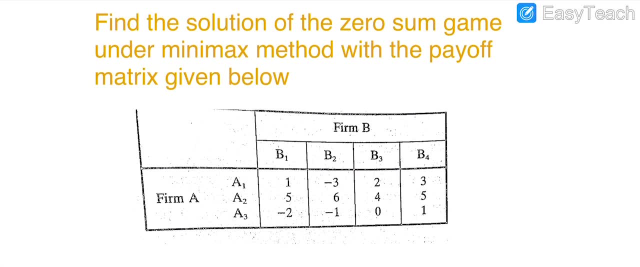 sum game can be solved. uh, when two forms are playing actually zero sum k? uh, same game can be solved with the help of two types of methods. first we see minimax method and then we see dominant method. so first we are going to solve zero sum game with the help of minimax method. 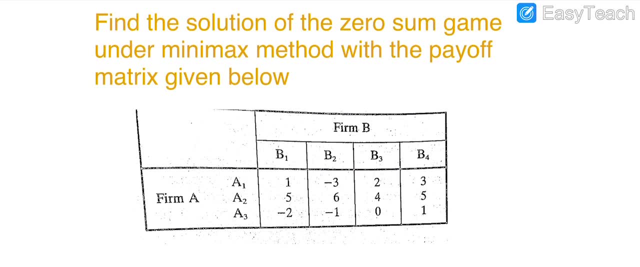 what is minimax method before its definition? you can see here below table is given and this table show two types of forms, from a and from b. uh, see here that from b having four options: b1, b2, b3 and b4. these options are actually the. 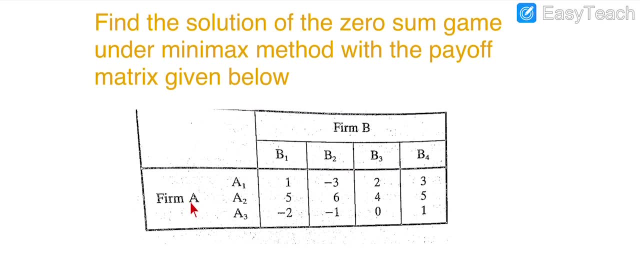 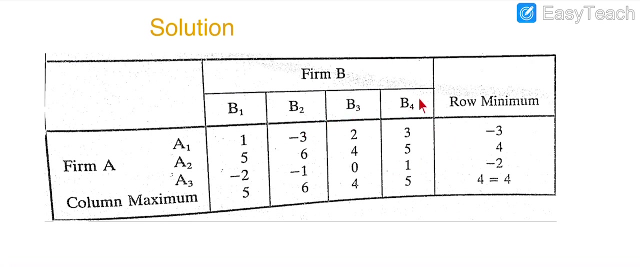 strategies which form can adopt and from a has three options: a1, a2 and a3. these are actually strategies which form a can adopt. you have to see this how we have to solve this table with the help of minimax method. let's see here: this is the solution. when you have to find, uh, the solution like this: then from a 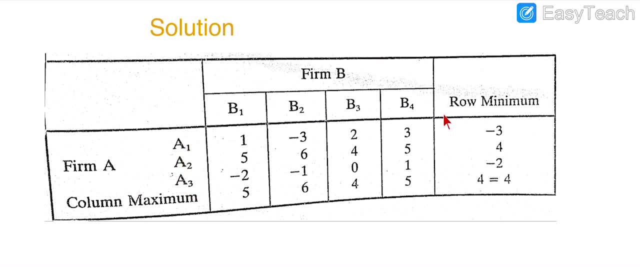 we have three strategies and from b have four strategies. you have to solve the problem that you take the maximum values column wise, what is columnized like this, column wise, and take minimum value row wise for c. you take first column one, colon5 v9c9-. 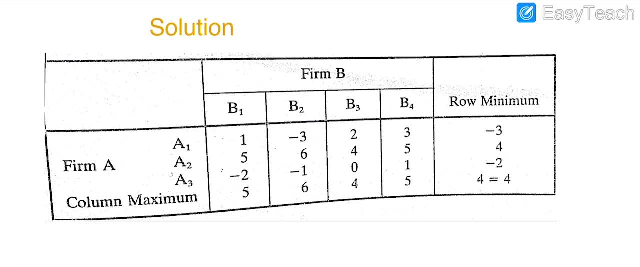 two. you take first column like this- i explained you till here. this is a1, a2 and a3. actually a1, a2 and 3. these are the three values: 1, 5 minus 2, and from the first column you have to take the maximum value. what is the maximum value? 1, 5 and minus 2, which is the biggest value. 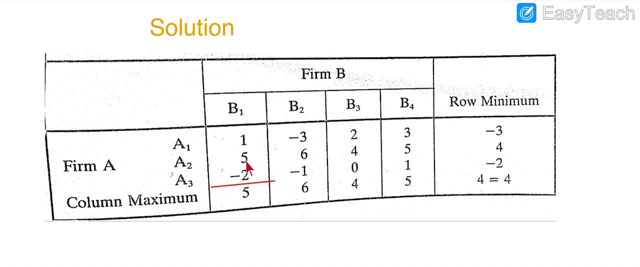 among these three, biggest value is 5. biggest value is 5. so you take it 5 clear from the first column, from column wise. you have to take the maximum value from this column. you take the maximum value, that is 5. next, if you see, see, in the second column, in the second column, you have to take the maximum value minus 3, 6 and minus. 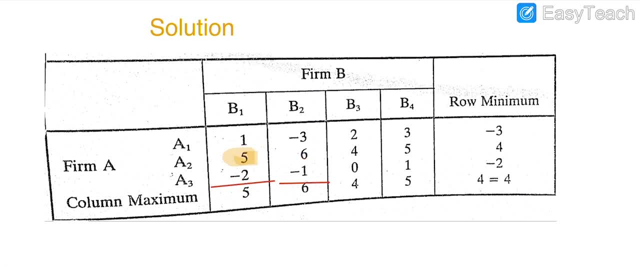 1, which is the maximum value. 6. understand: from each column you have to choose the maximum value. clear. in the next column you see 2 4 0, 2 4 0, which will be the maximum value among 2, 4 and 0, which. 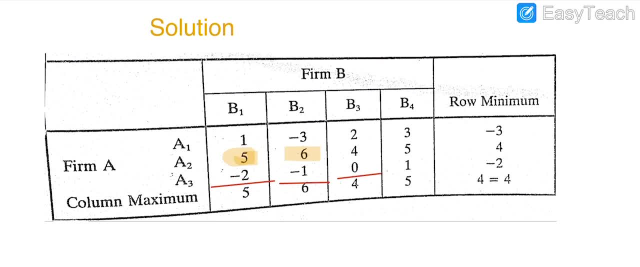 will be the maximum value, that will be the 4, clear. and what will be the next from the forced column? what will be the maximum value? if you see it, form 3, 5, 1, which will? which is the biggest value? of course, it is the 5. yes, now you can see we have a range of 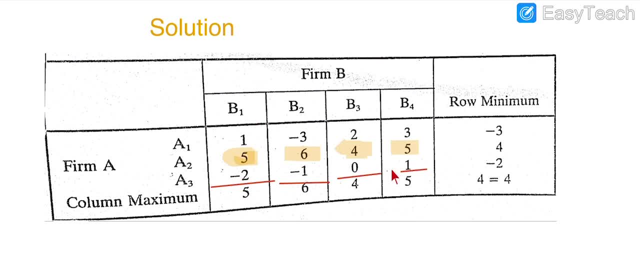 which is the biggest value? of course it is the 5. yes, now you can see we have a range of the columns and from all the columns we have taken out the maximum value you have to any in the columns through with the help of maximum. so arrange the column maximum value, column maximum you have. 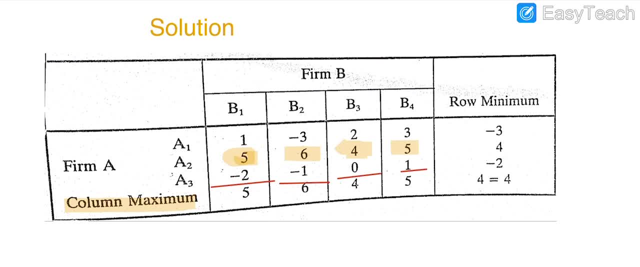 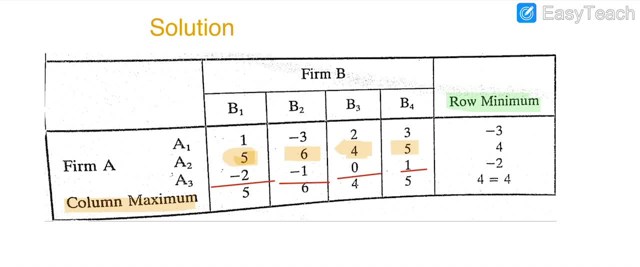 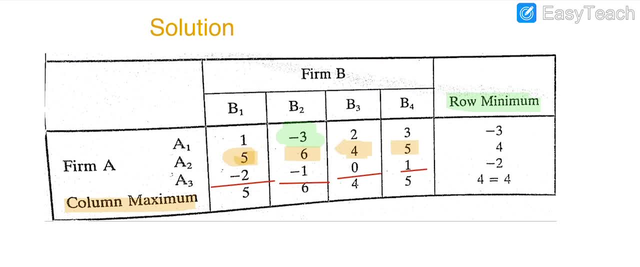 four. yes, it is the four. four is the minimum value. yes, from third row, you can see minus two, minus one, zero and one, which is the minimum value. minus two. minus two is the minimum value. yes, so how you have to find the solution. this is the main thing. do that's the need. 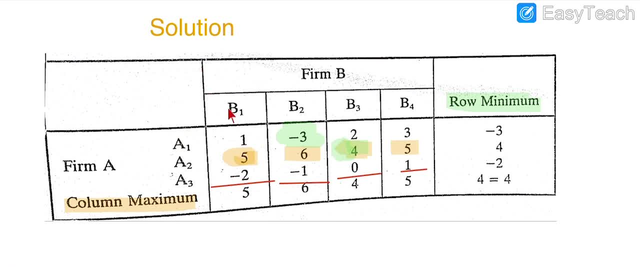 you have to understand, when you have done all this work, that you have arranged column wise maximum values and you have arranged row wise- minimum values. now you have to find the solution. you have to take that value which is common between the both, between the maximum column and between the row- minimum row, if you see.